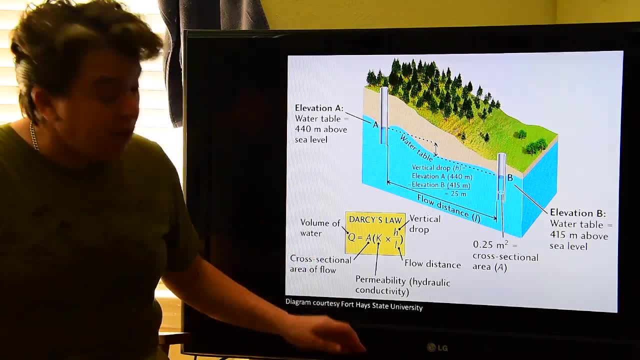 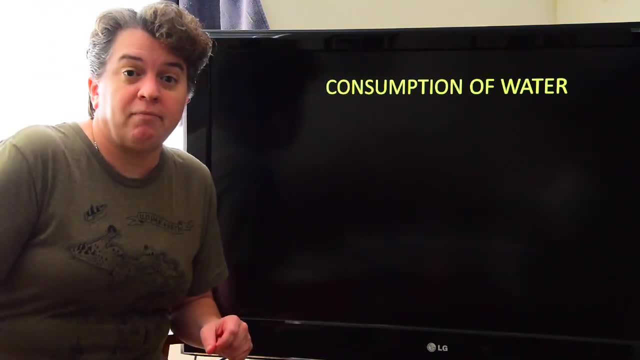 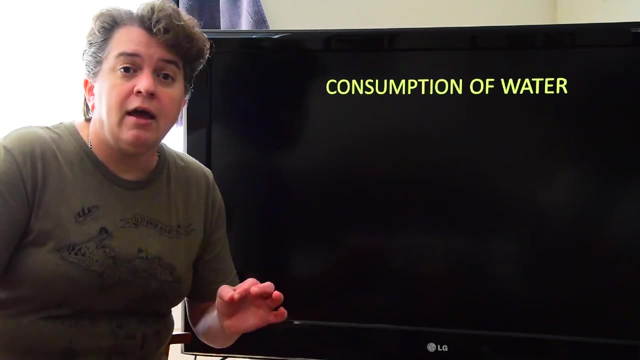 So see what you guys have to look forward to when you go to grad school. But anyway, let's move on and look at a little bit more about our water resources. So I said, one of the reasons studying and understanding and understanding groundwater is important is because we use it all the time. 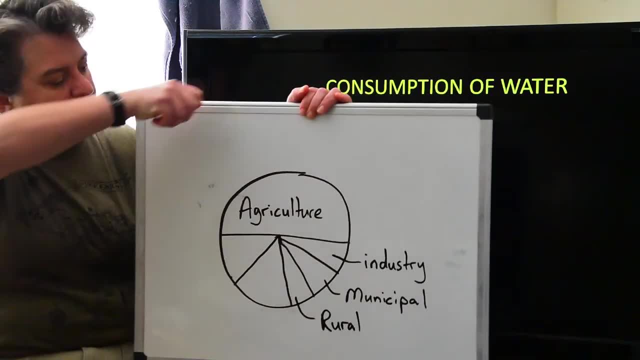 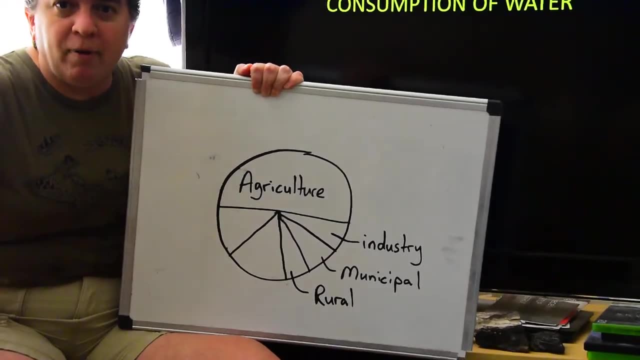 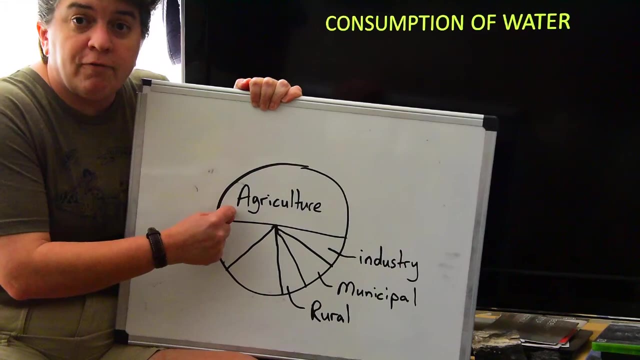 We use it for all kinds of different things. So the consumption of water in the United States. This is a very rough little pie chart, but it gives us a good idea. Notice, most of it is for agriculture, for farming, And that's basically you're going to be thinking. 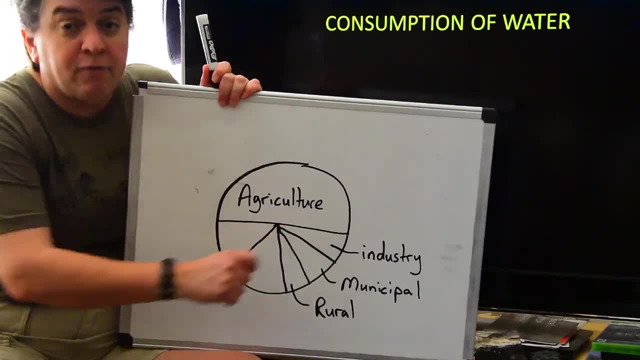 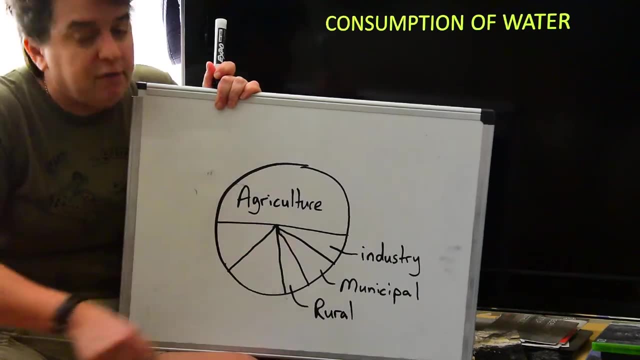 what is irrigation of crops and things? This little sliver is industry, So things like oil refineries, chemical plants, factories, stuff like that. Municipal, that's cities. So if you get city water, well, that's municipal. 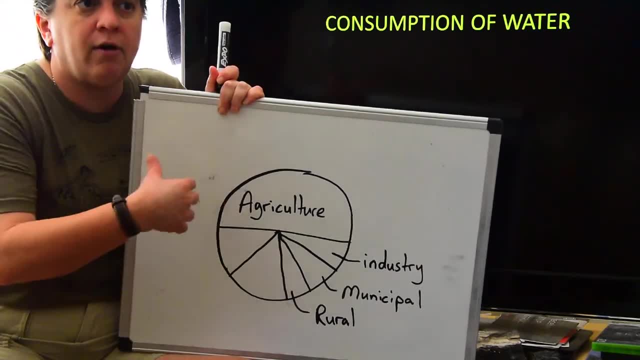 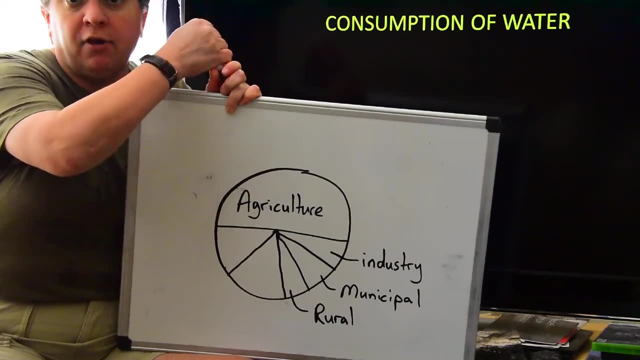 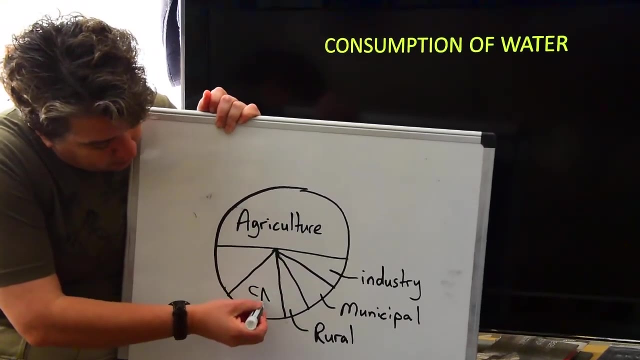 Rural means. this is not used for like irrigation or livestock. This is just if you have a well, for your own personal use. So that leaves us with what are these two things? Well, this here is California, Or, as Arnold Schwarzenegger would say, California. 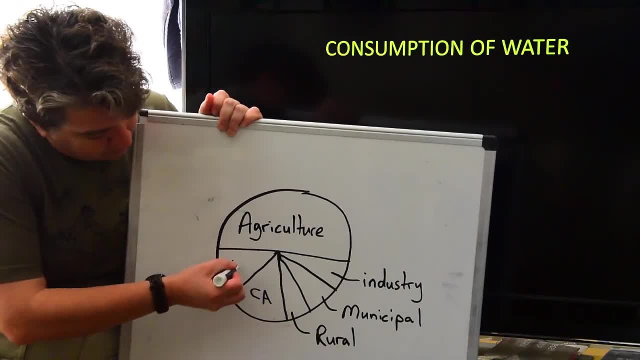 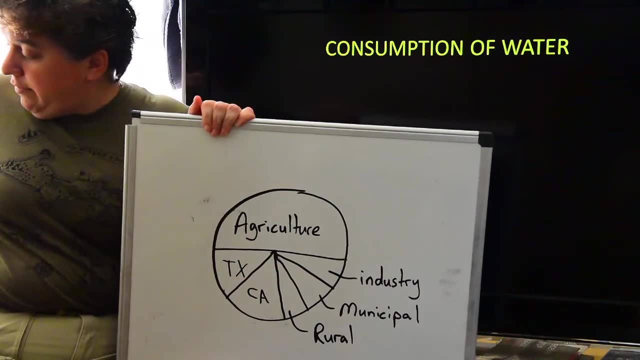 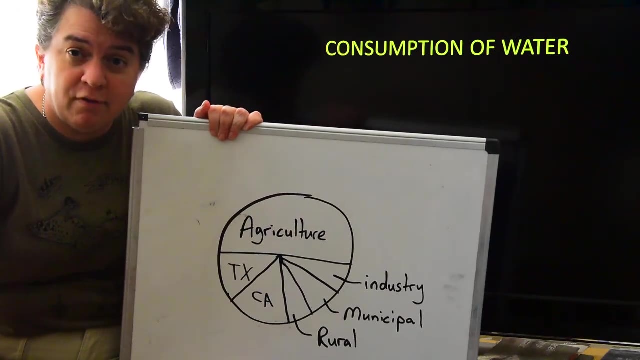 That's California, But this is Texas. So what this is showing you? those two places use a whole lot of water. Now, why do they use so much water? Well, they're big states with big populations, but they also have a lot of agriculture in them. 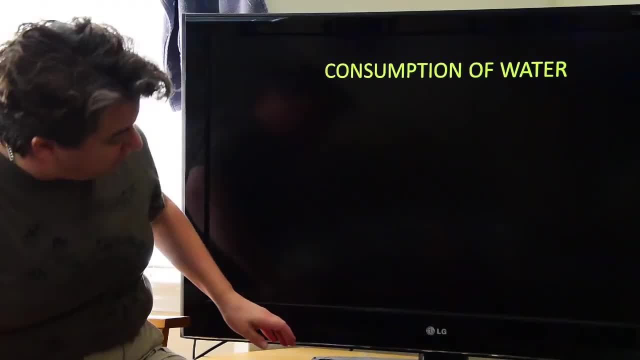 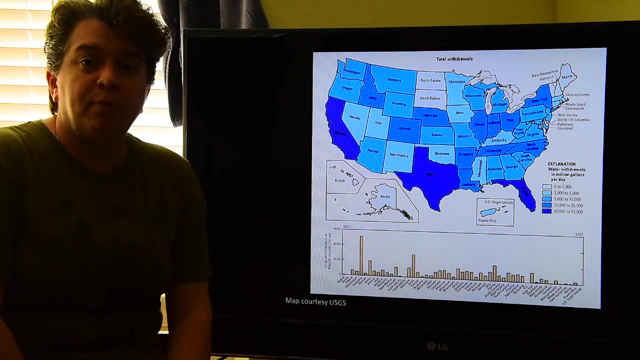 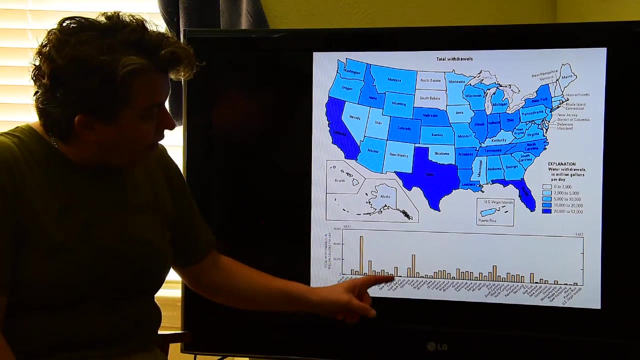 So water use is not the same throughout all the United States. This is just another way of looking at, kind of what I had in the big pie diagram. The darker, the blue, the more water is used, And here you can see a bar graph of the different states and how much water. 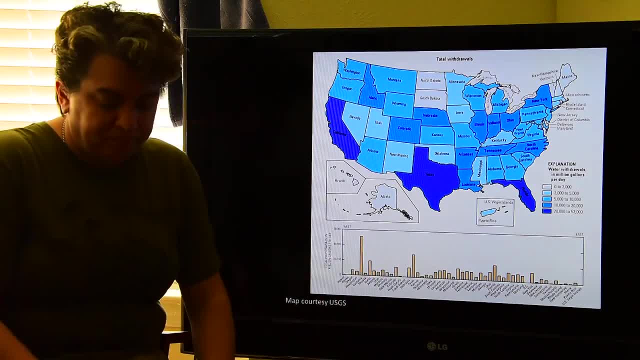 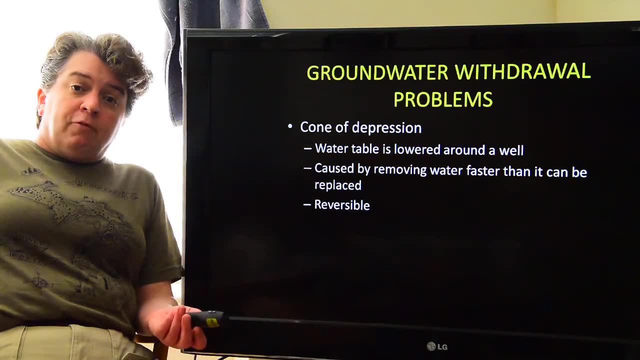 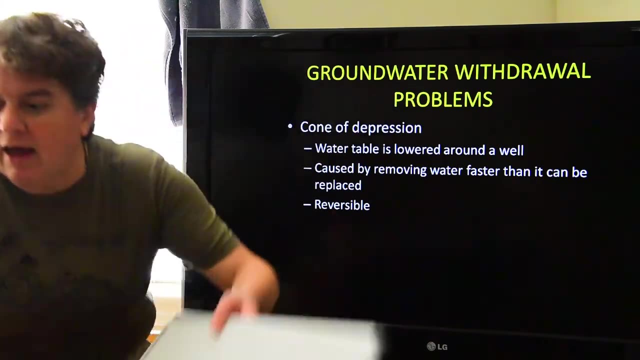 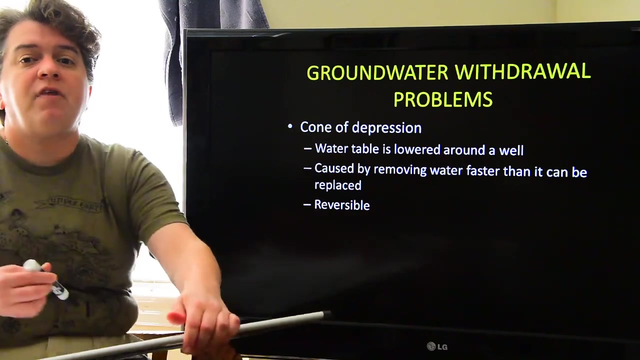 There's California, there's Texas. Now, when we use a whole lot of water from these different aquifers, there are some issues that we can end up having occurring, And one of these groundwater issues that can happen is something called the cone of depression. which sounds a whole lot like what my dog used to say. My dog used to have to wear when he'd come back from the vet, But the cone of depression is actually a groundwater problem. So let's start with a very basic aquifer. 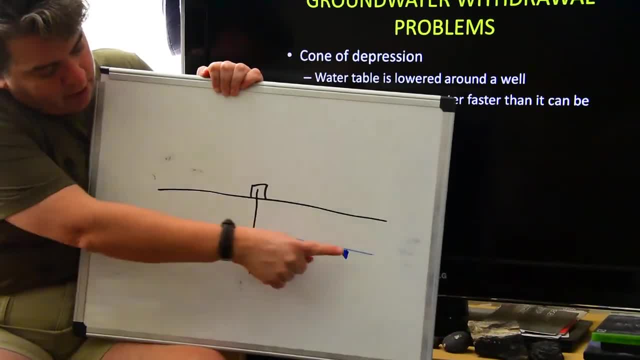 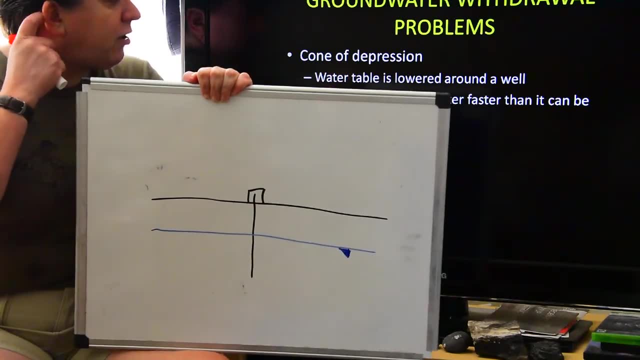 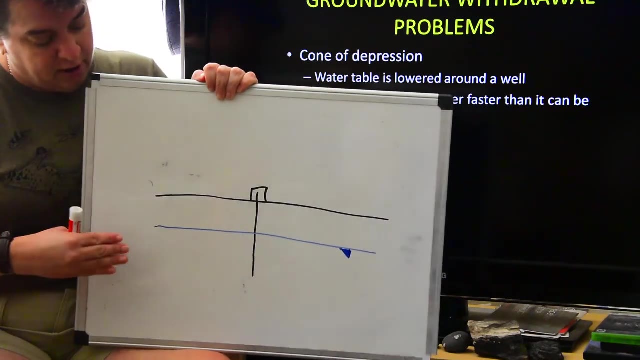 So here's Earth's surface, There's my well going down, There's the water table. So I'm taking water out of this aquifer And a cone of depression occurs when more water is removed from the aquifer and it's removed faster than it can be replaced. 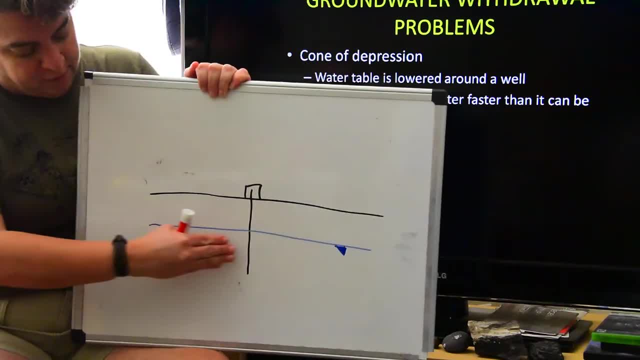 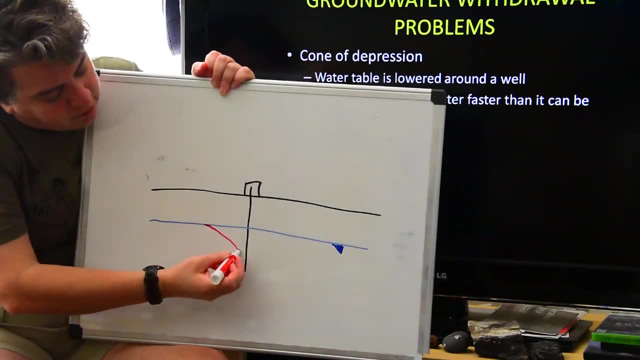 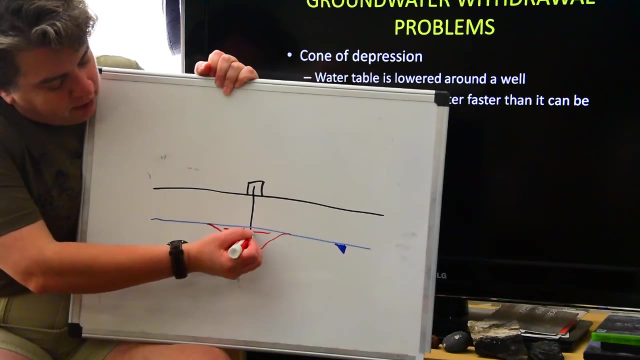 So, basically, we're pulling water out of that aquifer faster than it can flow back into that area. So what then happens is this water table around the well gets lowered, So all of this area that used to be filled with water. 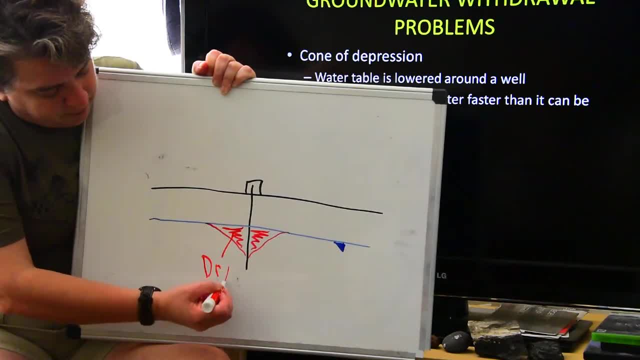 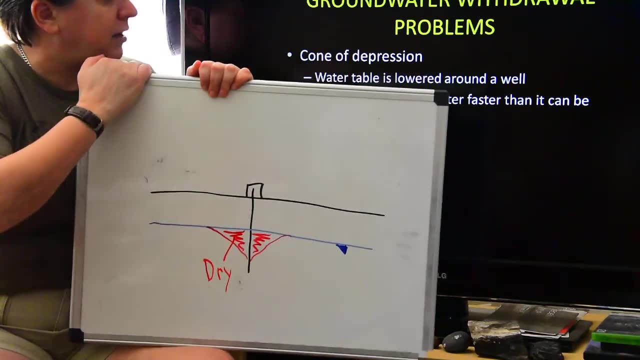 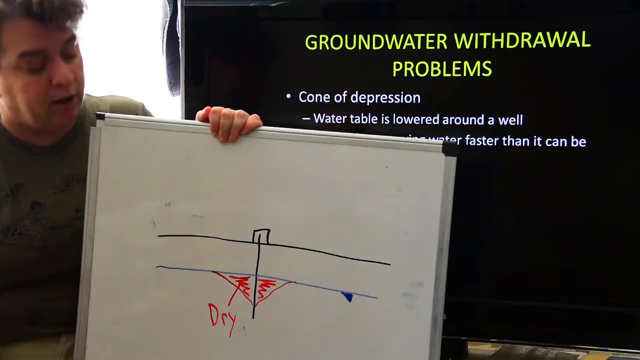 all of that is now dry, So we're taking out this water faster than it can be replaced and slowly that water table is going to get lowered around the well. I know it looks like the triangle of depression drawn here, but imagine that in three dimensions. 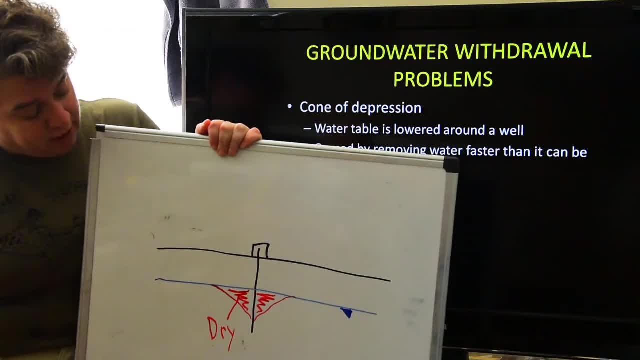 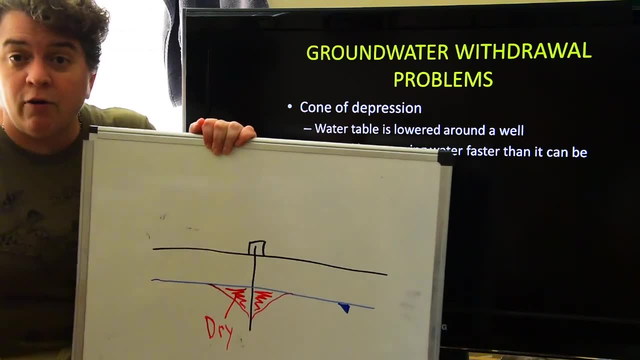 It's a cone And this can be bad, because this actually can make other people's wells go dry. What if you had a neighbor whose well wasn't quite as deep? It might go dry, But there is good news about that cone of depression. 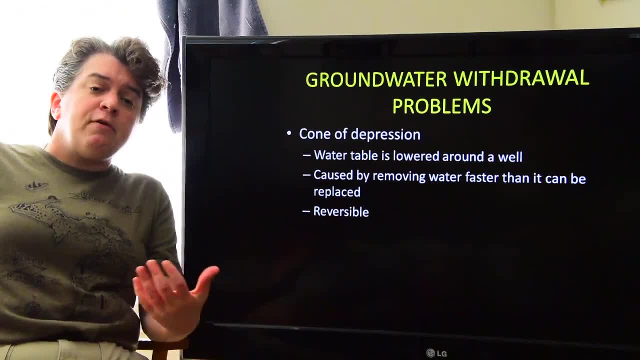 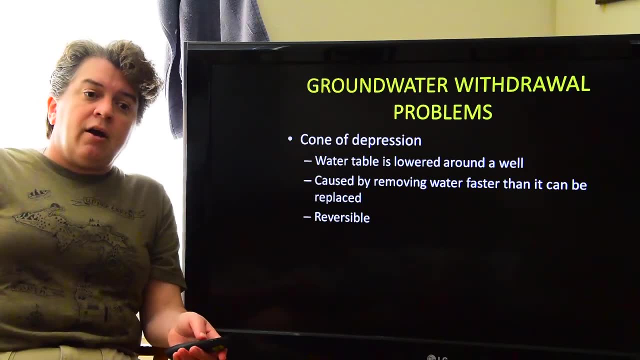 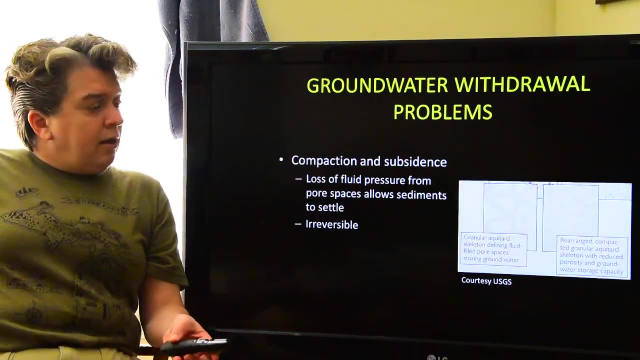 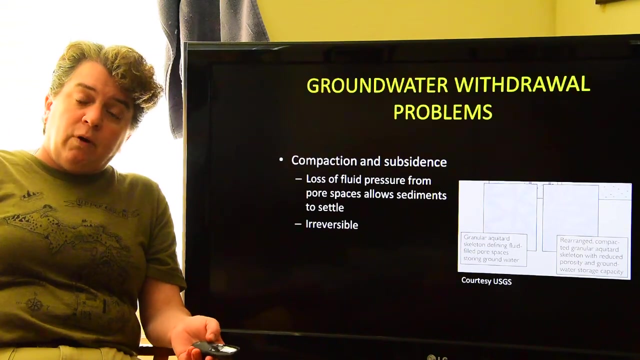 It's reversible. If you start to conserve your water usage, don't use quite as much water anymore. the water then can recharge the area and the cone of depression will be solved. Unfortunately, there are there are issues that are irreversible when we use a lot of groundwater. 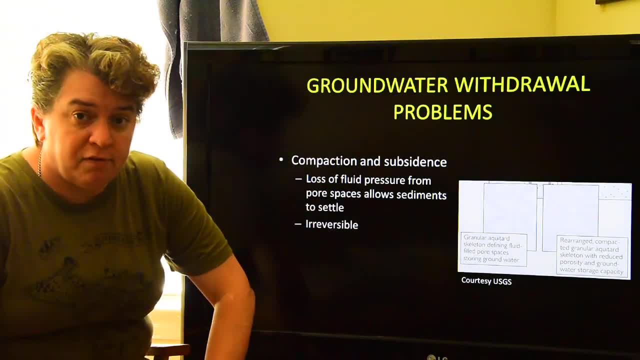 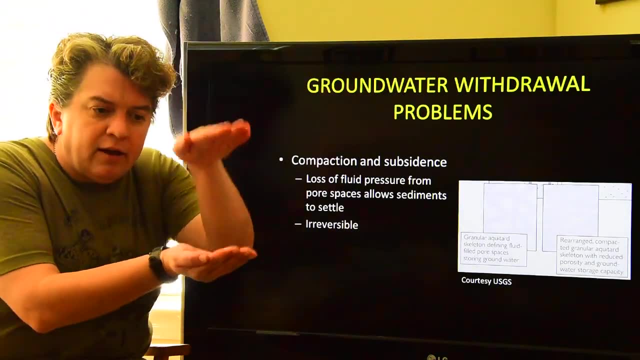 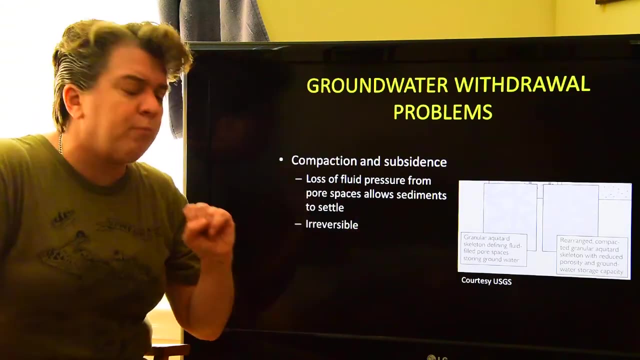 One of these is compaction and subsidence, And so compaction is when sediment gets like squeezed closer together, And this can happen because of this loss of fluid pressure from pore spaces. Okay, We know that like gravity pulls stuff down right. 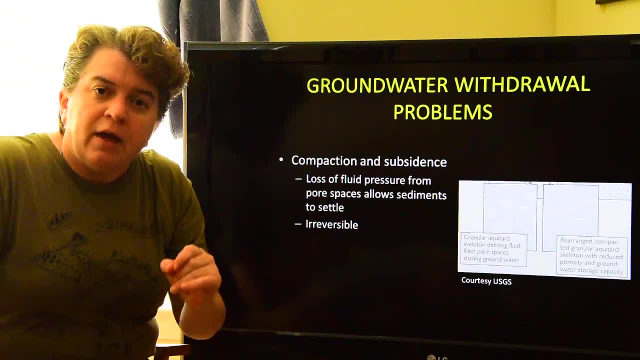 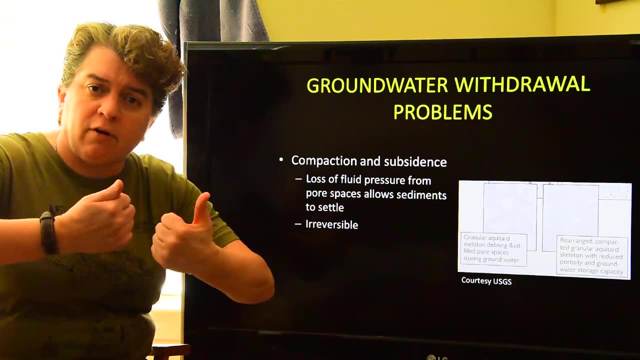 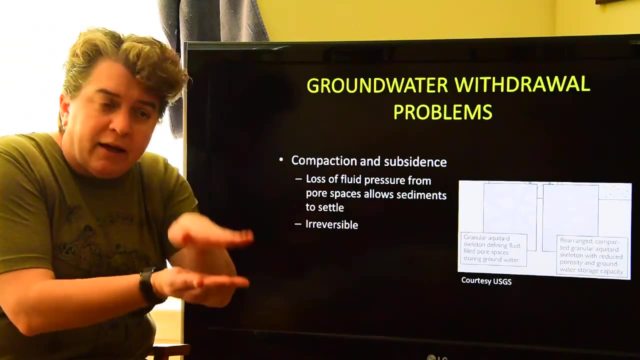 And so sediment wants to kind of squish together, But water, being a liquid, is not compressible, So it actually exerts a force called this, this pore fluid pressure, that keeps the sediments from packing really really closely together, And that's what we're trying to show here. 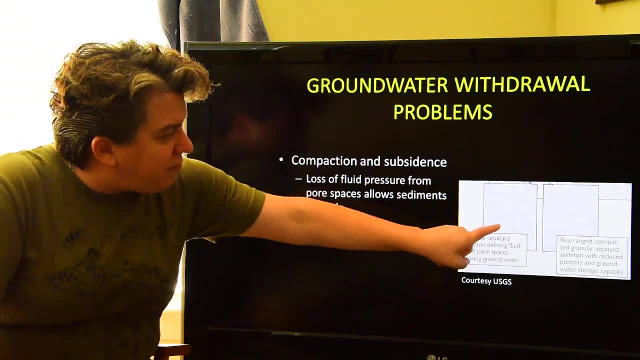 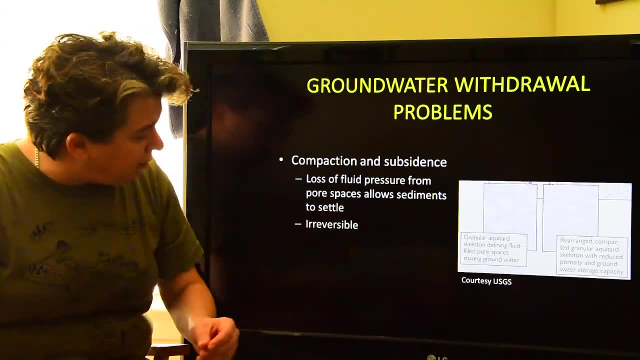 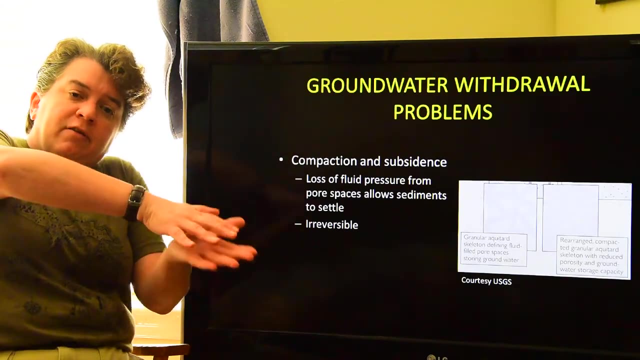 We have these spaces in here. These spaces in between the little grains of sediment are filled with water and preventing that sediment from squishing closer together. But if we remove that water then this allows the sediments to compact and settle much, much closer together. 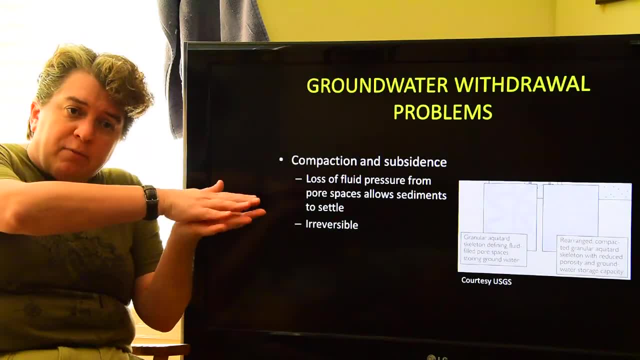 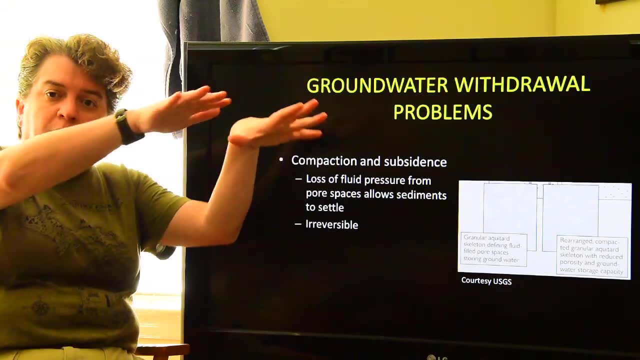 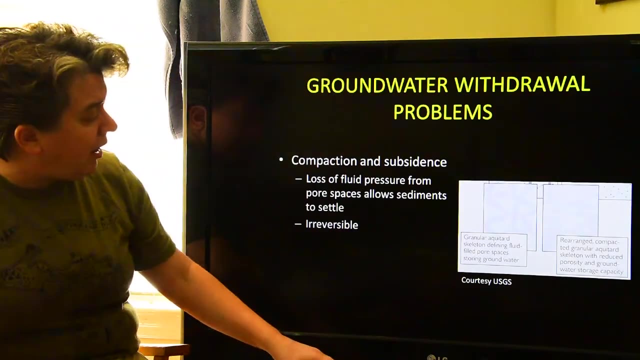 And what this does, then that's the compaction, The sediments kind of coming closer together. Subsidence is where the entire earth's surface above this area will actually sink. It will get lower in elevation And this is irreversible. 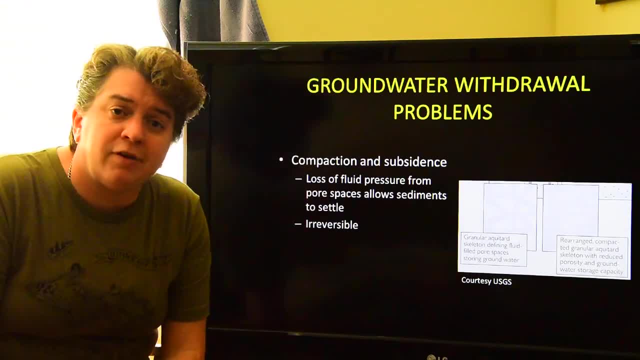 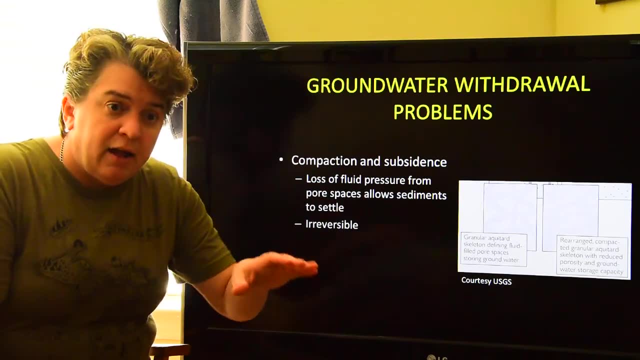 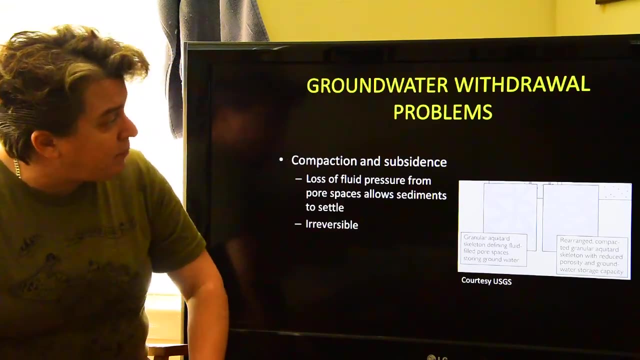 Once those sediment grains pack closer together, it's not like you can pump water down there and re-inflate it or something. Once that's, they settle. all of that porosity that was once there is gone forever and cannot be gotten back. 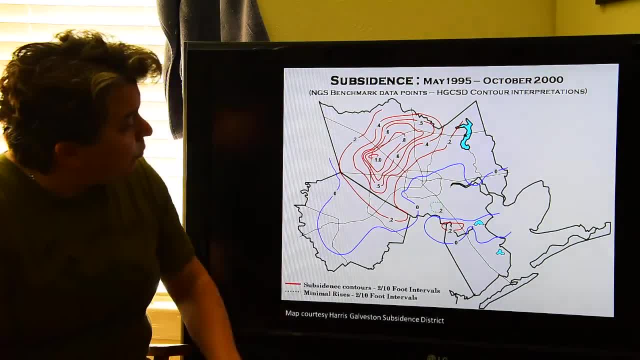 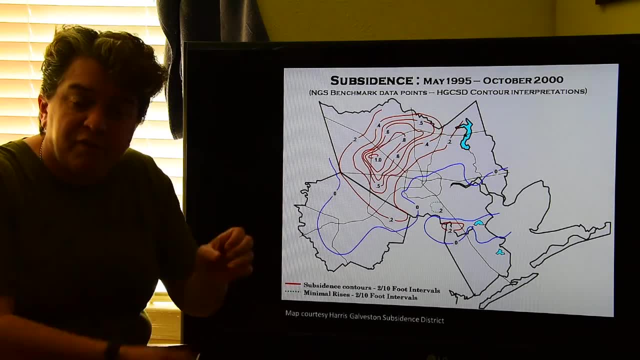 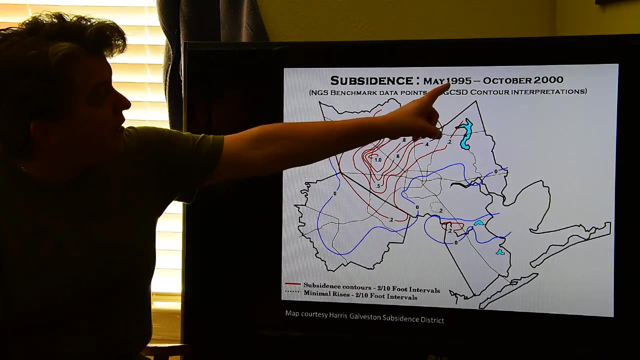 So this is something that occurs closer to home. We can see this is the Houston area And this is subsidence caused by this compaction of sediment because of the withdrawal not only of water but also of some oil in this area. But this is just five years, from 1995 to 2000.. 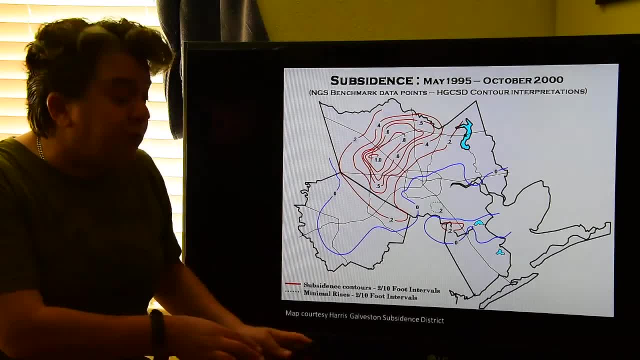 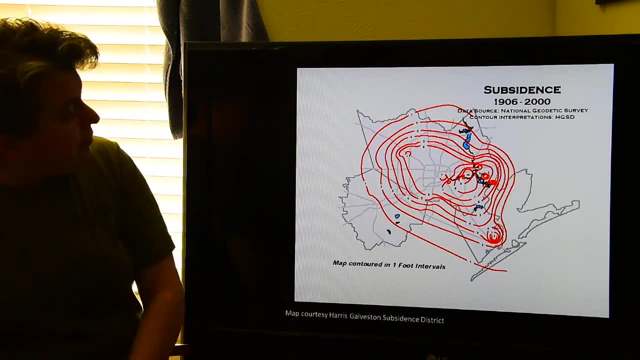 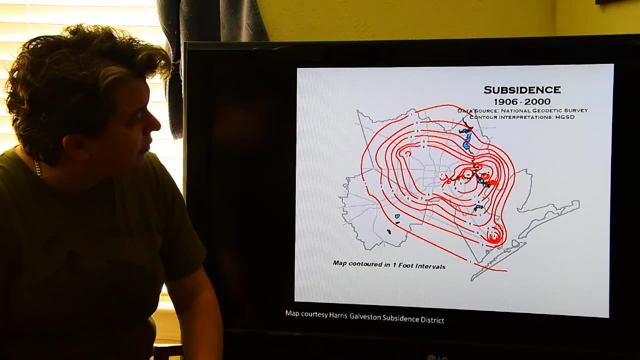 You can see some areas subsided afoot. That means the surface elevation lowered that much in five years. It gets even worse if we look at the subsidence over close to a hundred year period from 1906 to 2000.. And these are in feet. 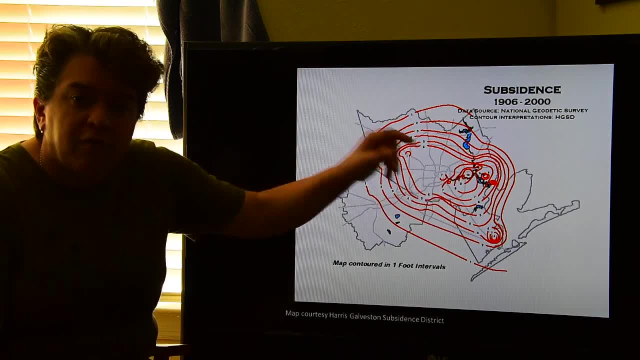 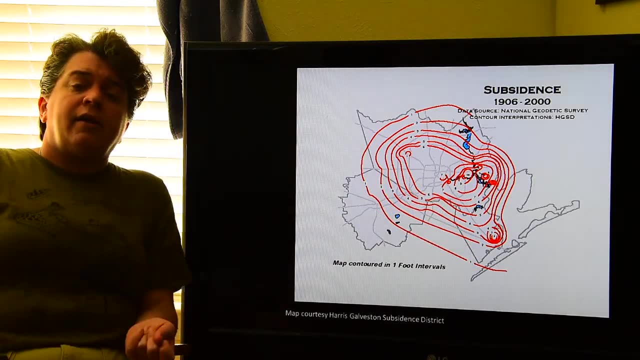 And you can see some areas. there's ten feet of subsidence And these are actually right near Galveston Bay as well and the ship channel, And so these were close to sea level anyway. And then you subside them ten feet, they're suddenly under sea level. 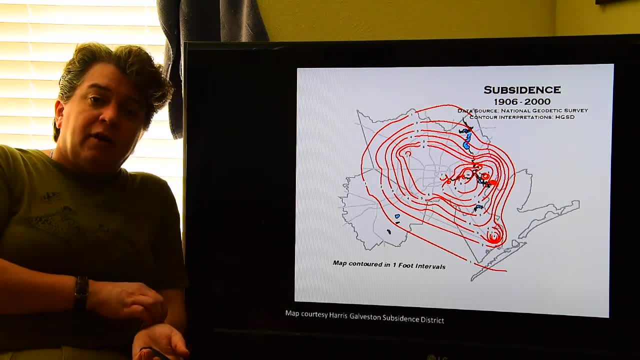 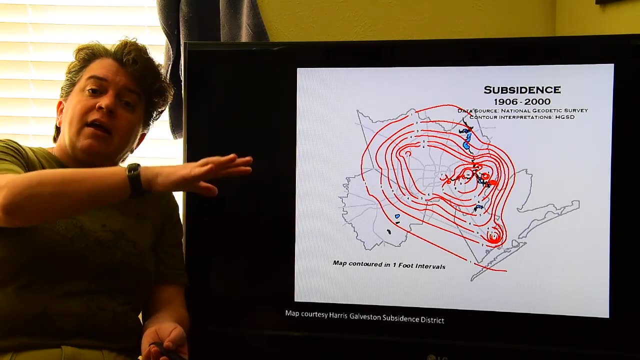 In fact, there is an entire subdivision here in the Houston area, somewhere out here, that had to be abandoned in the early 1980s because when it was built it was a few feet above sea level, and then it subsided below sea level. 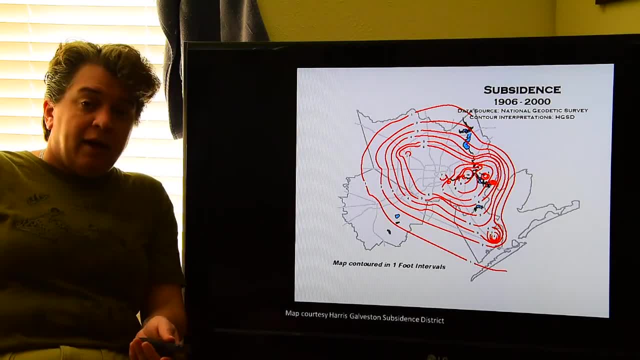 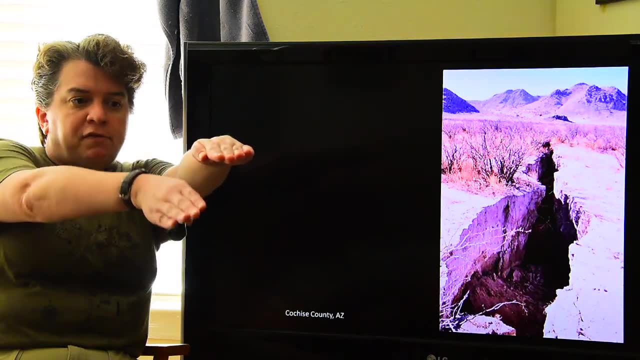 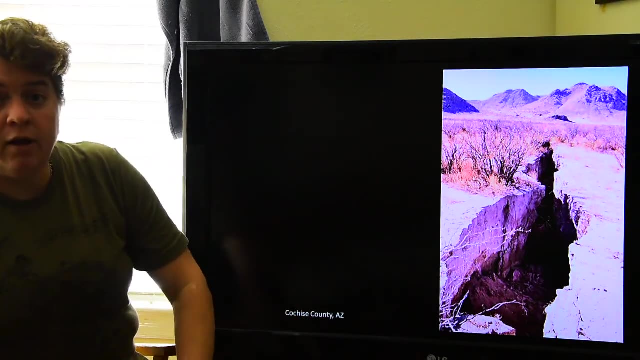 and became flooded and everyone had to leave that area. When you have this subsidence, when you have areas that are sinking and then some areas around that are not, you can also develop these large fissures in the ground. These are seen in the area surrounding, like Phoenix Arizona. 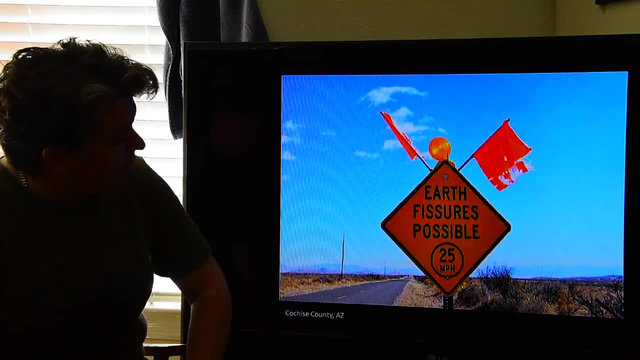 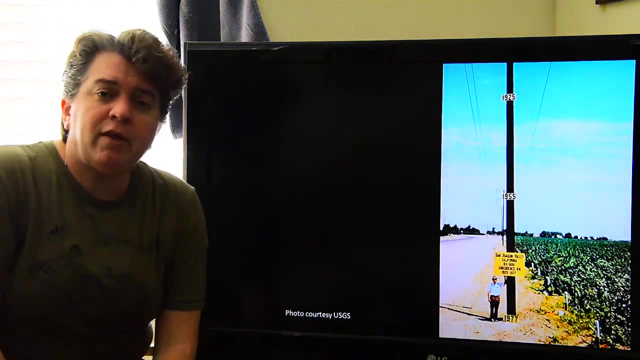 And you'll drive around and you might see some signs like that: earth fissures possible, though this was my favorite one with the little car like that. But probably the most famous place that's had subsidence is the San Joaquin Valley in California. 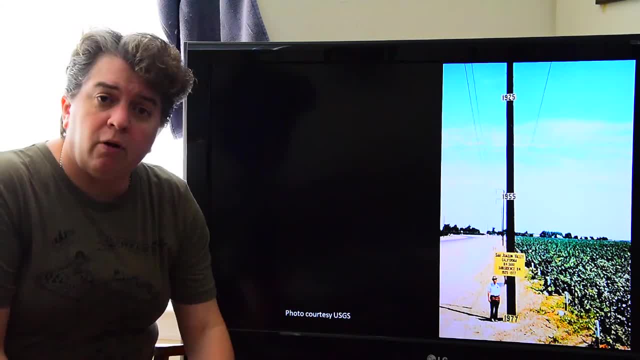 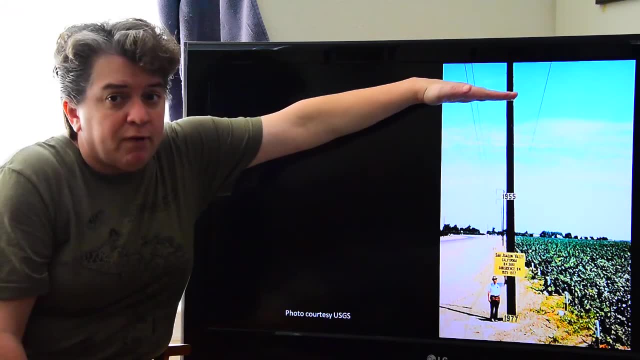 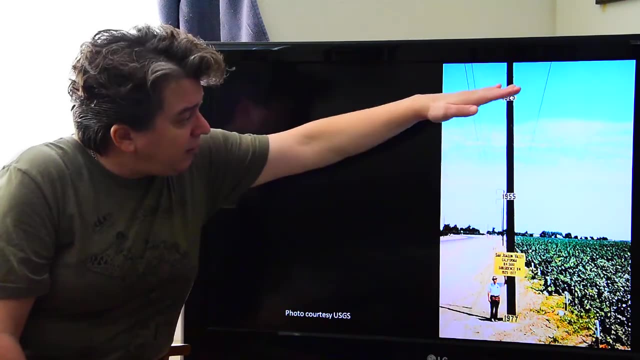 It is a major agricultural area. They withdrew a whole lot of groundwater to irrigate crops And we can see: in 1925 the land surface would have been up here, And by 1977, just what 52 years- the land had dropped that much. 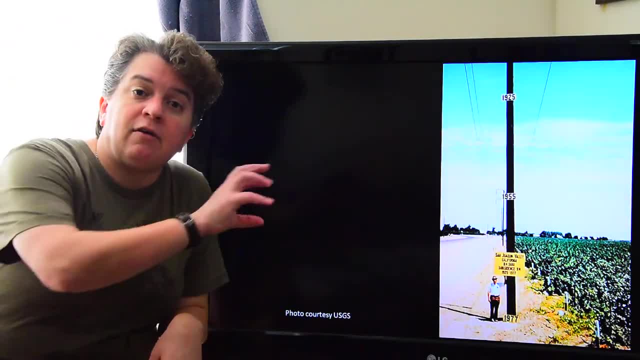 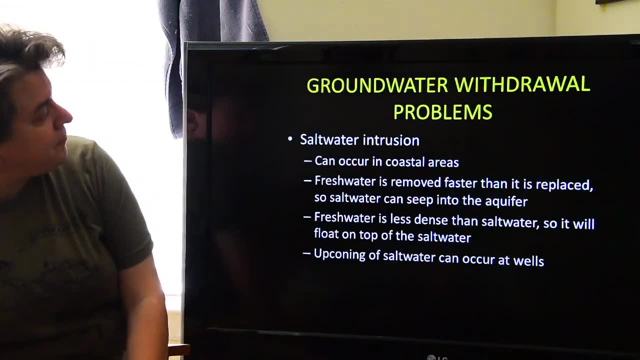 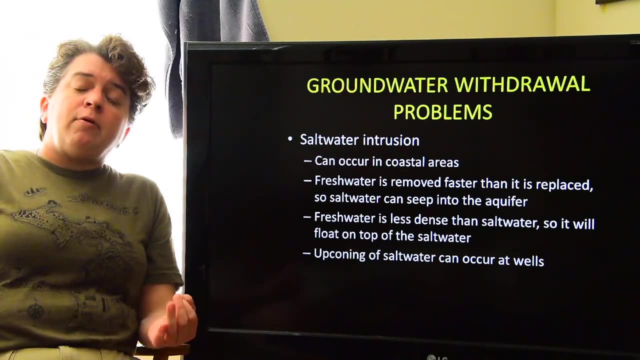 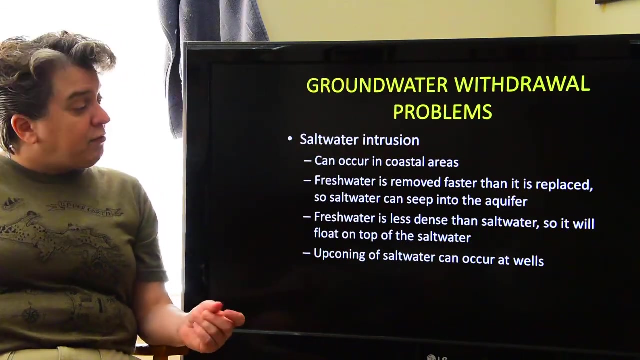 And all of that is lost. porosity- That is all area that water. once occupied underground, All right. there are other groundwater problems. Saltwater intrusion is a problem that can happen in coastal areas, So we have to be near the ocean where we can have saltwater. 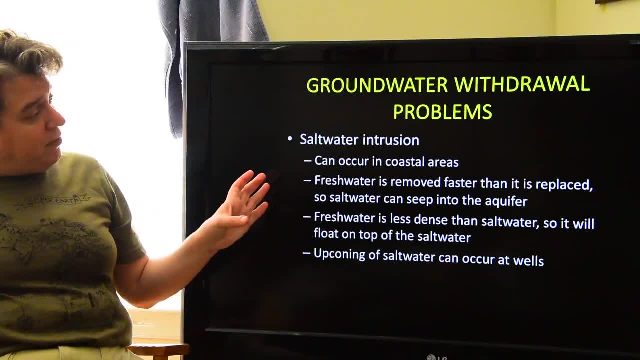 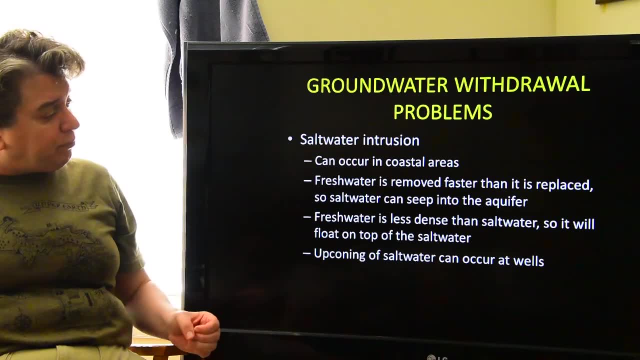 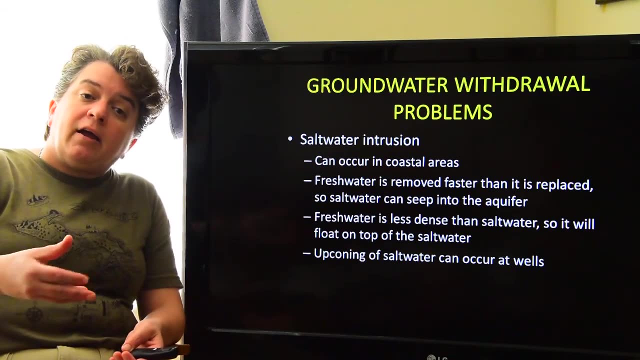 So what happens in areas where you have this saltwater intrusion? fresh water is taken out of the aquifer faster than it's replaced, So saltwater can then start seeping in into the aquifer and occupying area that fresh water used to occupy. 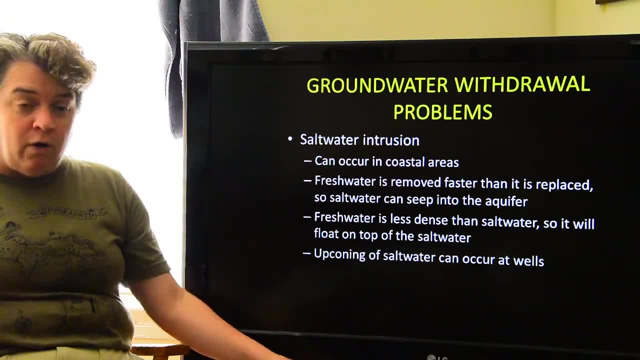 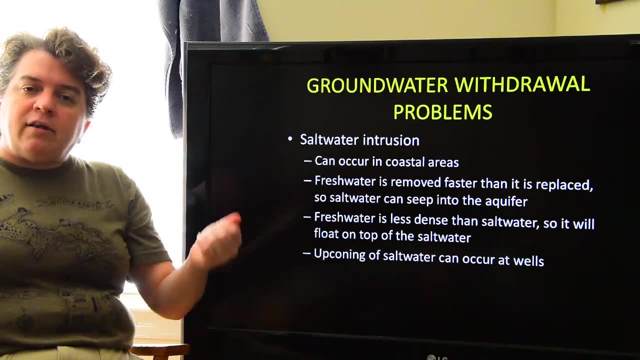 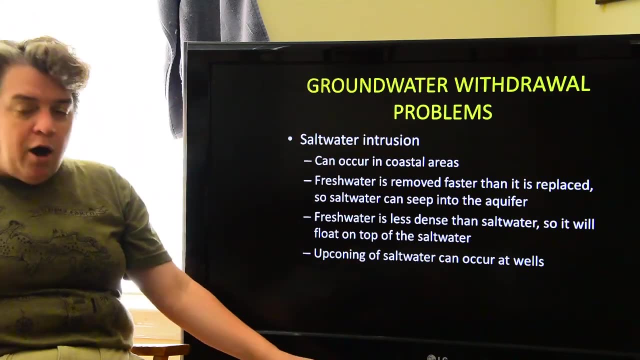 Now, fresh water is less dense than saltwater, So it will actually float on top of the saltwater, But as you start extracting things from a well, the well basically sucks the saltwater upwards, And this is called upconing. So let's take a look at what's going on. 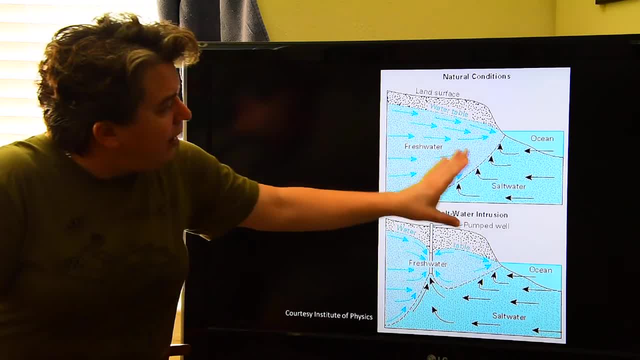 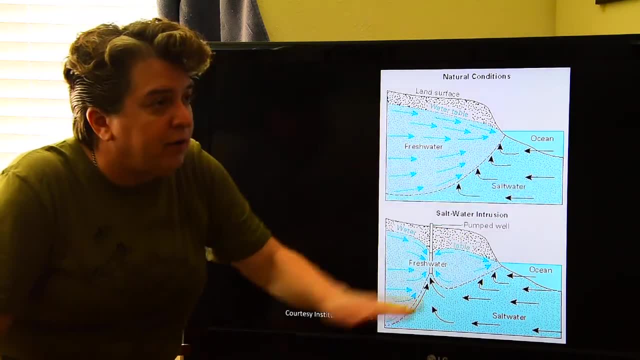 This is our natural conditions. We've got the ocean out here, We've got fresh water here. There's the land surface, Here's the water table. So we've got an area of fresh water and area of saltwater. But as we start extracting that fresh water, 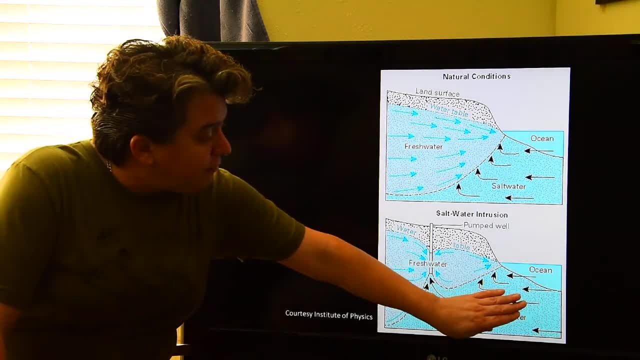 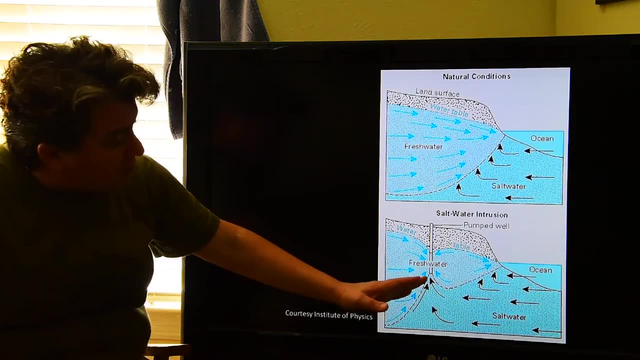 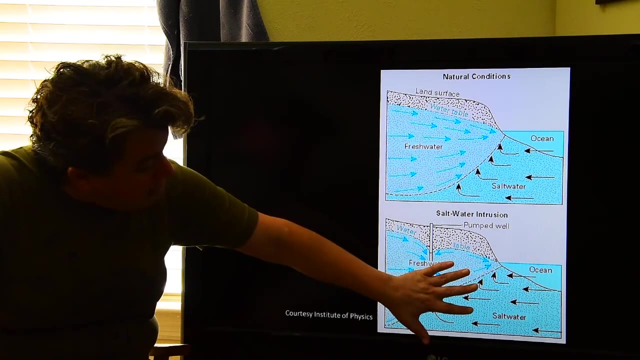 the water table goes down and there's more area for this saltwater to start occupying. So the saltwater starts entering areas where fresh water used to be, And as we continue to extract out of this well, we'll actually start pulling some of that saltwater into it. 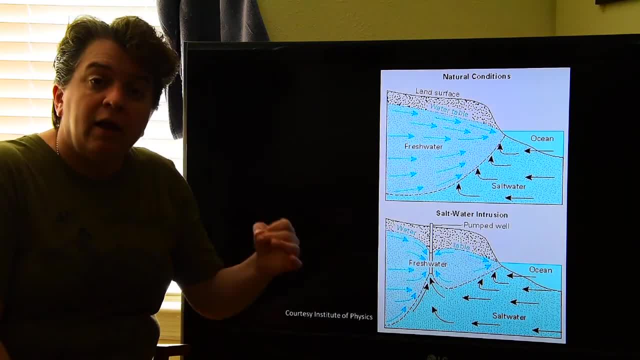 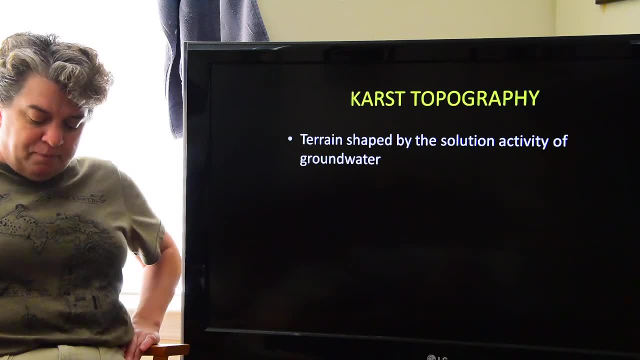 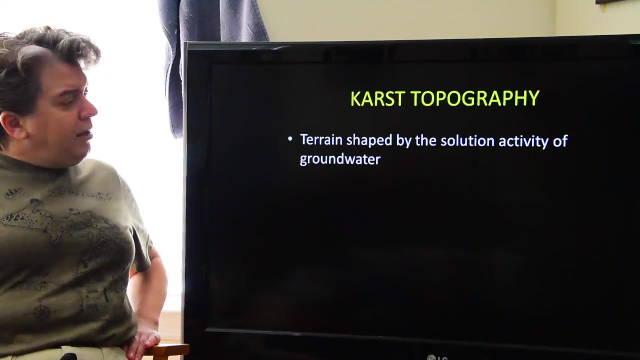 And so this is something you've got to be really careful about in coastal areas, All right. Well, usually in this class I have something about how Earth is trying to kill you, And, yeah, karst topography counts for that, But karst topography is also caused by saltwater. 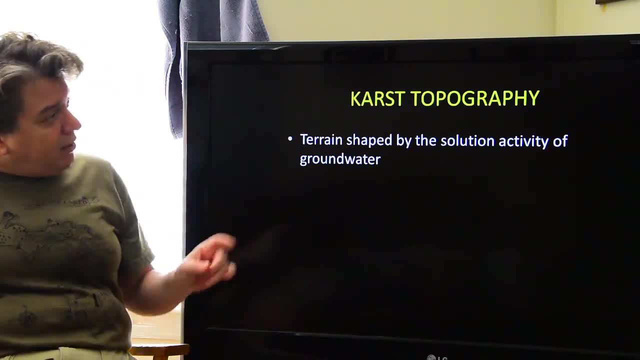 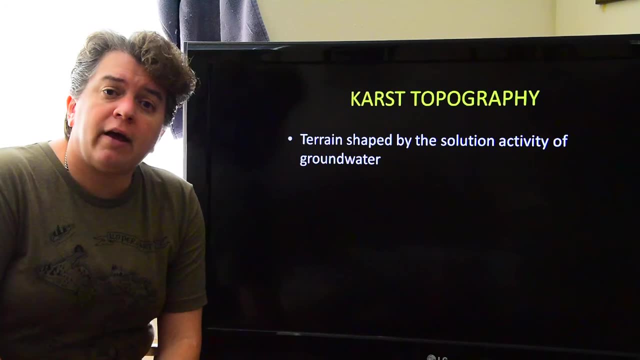 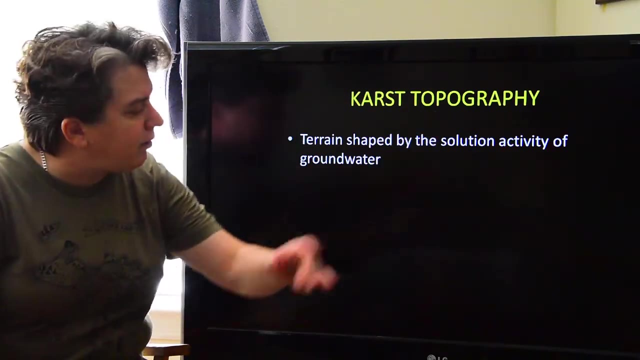 It's also caused by groundwater. Now, karst topography is a terrain shaped by the solution activity of groundwater. Solution activity meaning the groundwater is dissolving away, rock dissolving it and carrying it away, So this can only happen in soluble rocks. 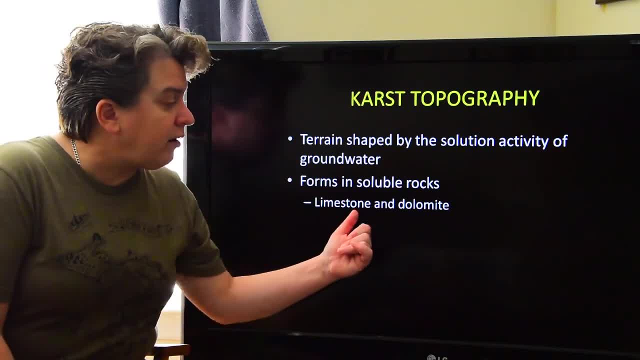 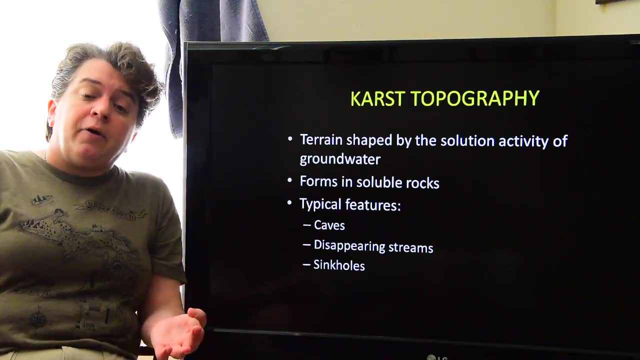 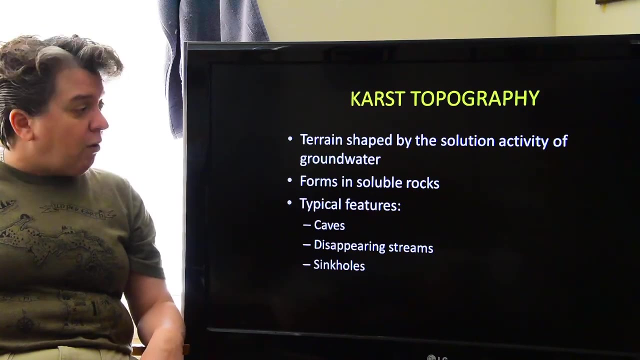 And the most common soluble rocks that you'll see are limestone and dolomite. Now, typical things that you'll see in an area of karst topography are caves, disappearing streams and sinkholes. So this is a diagram showing karst topography. 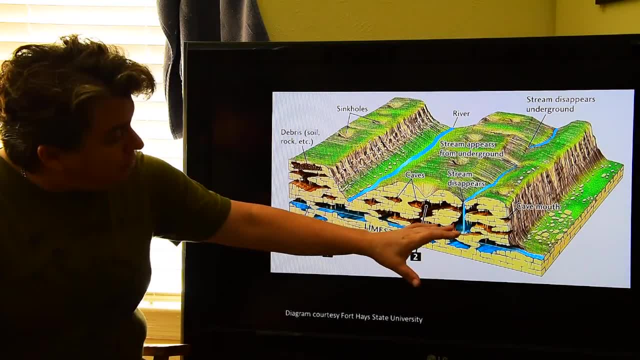 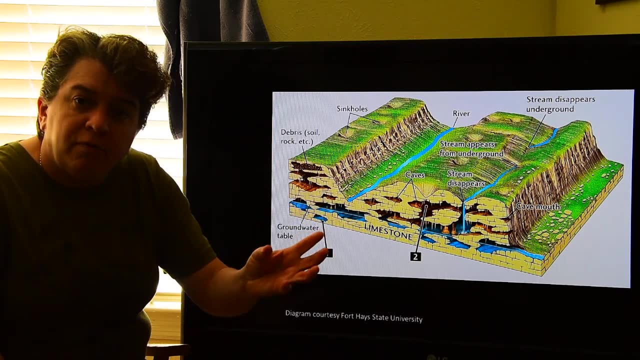 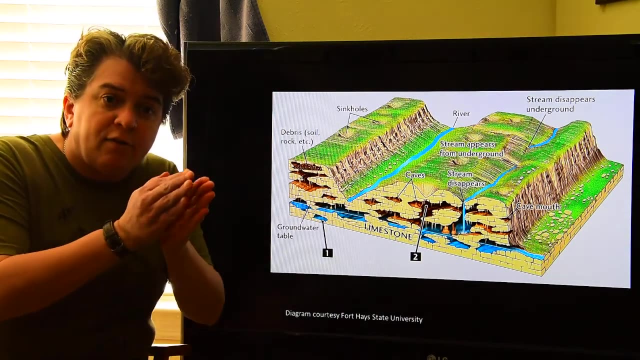 And these caves are these open areas that were formed as groundwater flowed through little cracks and little permeable parts of the limestone And it would dissolve away more and more of the limestone. So what began maybe as a small crack gets widened and it gets bigger and bigger and bigger and bigger over time. 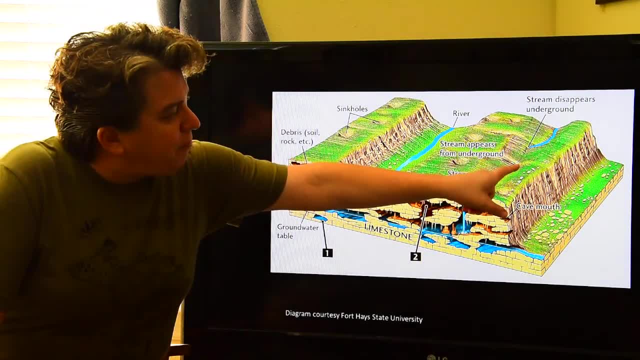 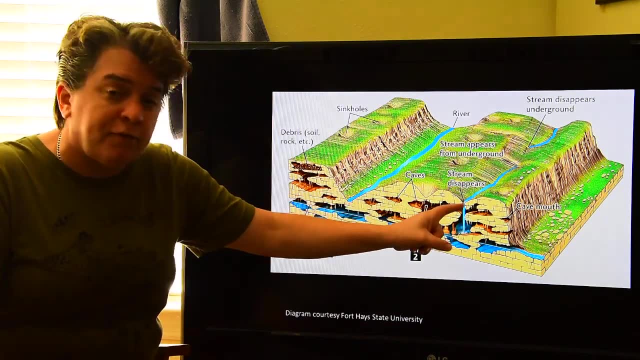 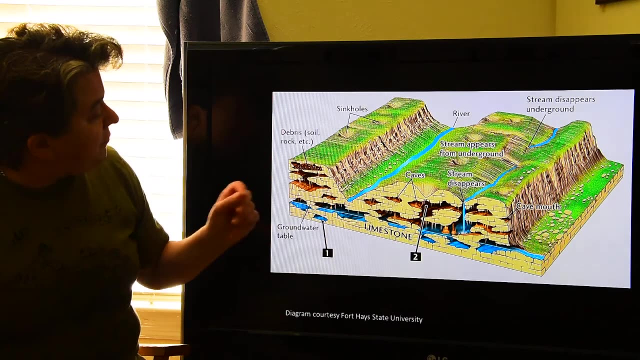 Disappearing streams? are these streams that pop up from underground? Basically, they flow out of a cave somewhere, They flow over Earth's surface for a short distance And then they drop into the subsurface, into another cave somewhere, And sinkholes form. 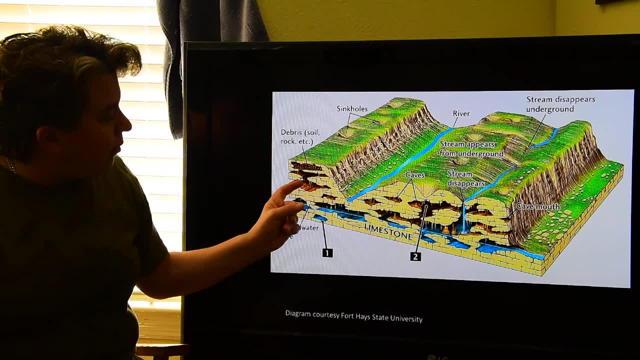 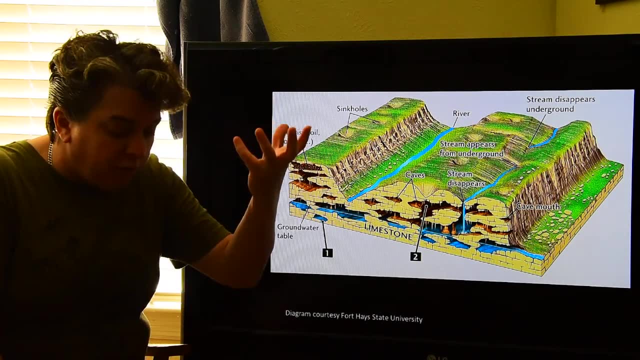 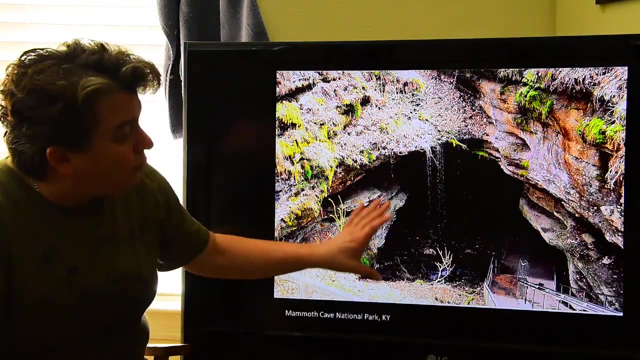 There are going to be these depressions that we get. They form where the roof of one of these caves got so thin that it could no longer support its own weight And it collapses. So this is a cave. Imagine all of this was once limestone that has been dissolved away by water. 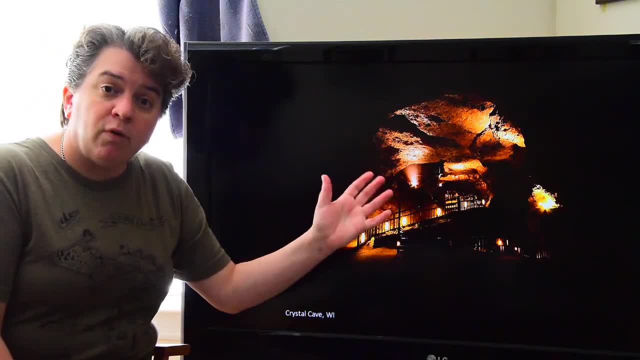 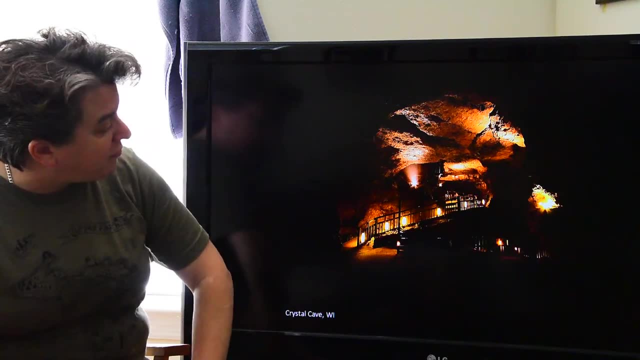 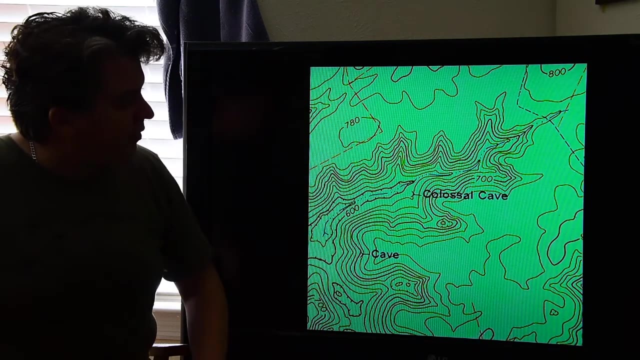 And this is underground in a cave Again. all of that once was rock. Over time, the rock was dissolved by groundwater, leaving this open space. This is a topographic map of a disappearing stream. We're looking at not more than about a mile. 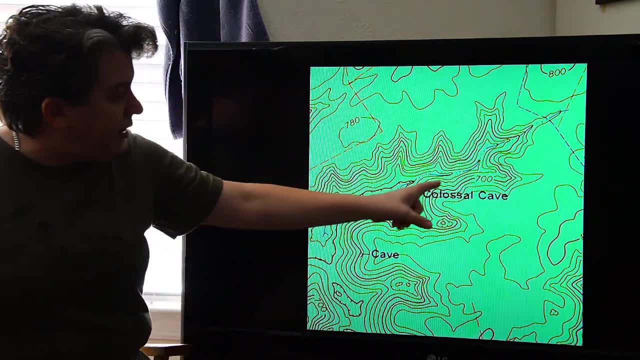 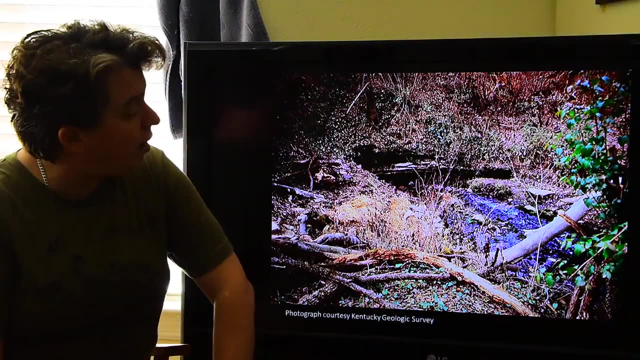 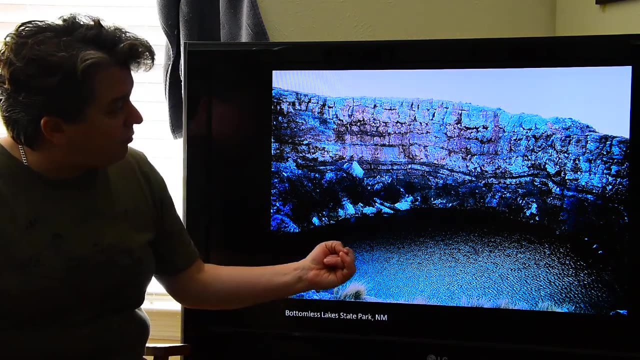 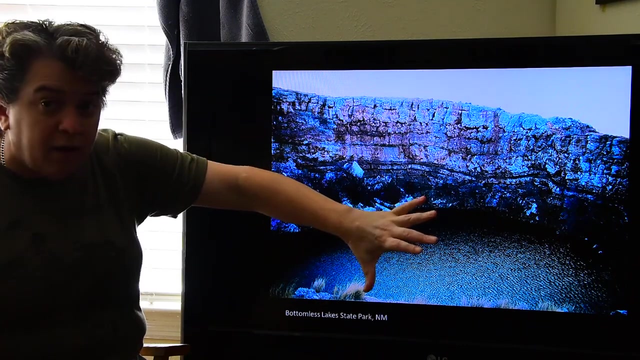 And we see the stream shows up right there. It flows and it disappears. This is a disappearing stream showing up on Earth's surface from a small cave, And then we have these sinkholes. So all of this, there used to be basically a roof over this covering this area. 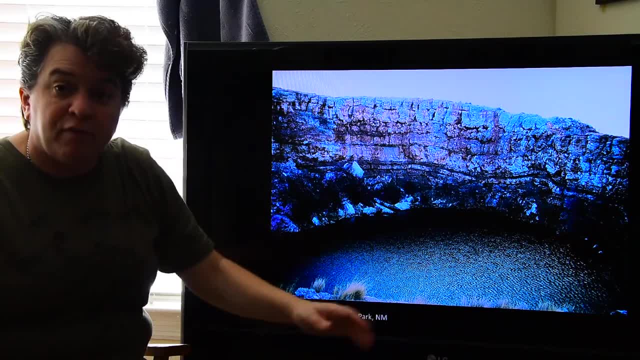 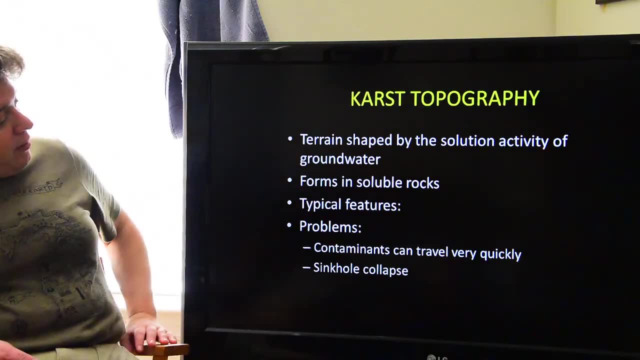 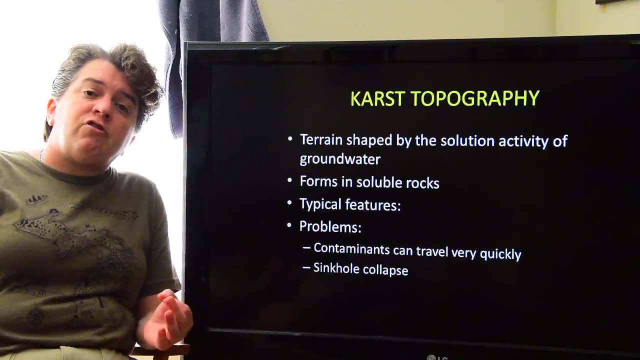 But that got so thin it eventually collapsed, revealing basically the cave system that was underground. So what are some of the problems associated with karst topography? Well, first of all, contamination can travel really quickly Because in karst topography you do have these caverns. 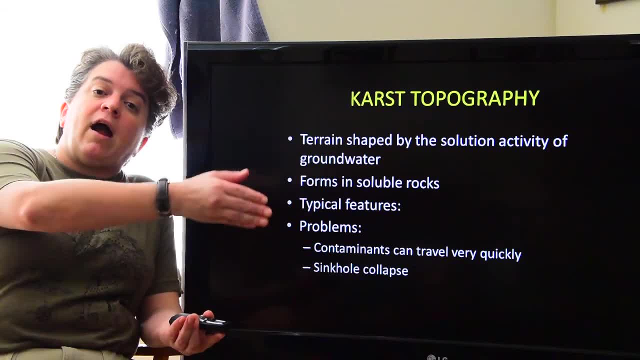 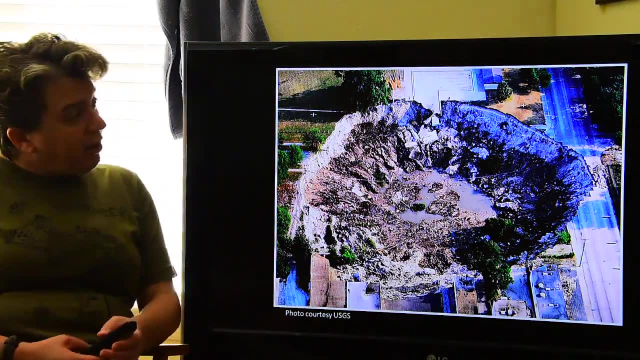 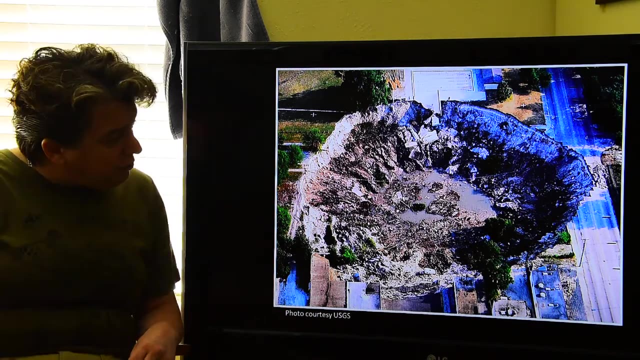 these open spaces where contaminants can rapidly travel underground. And then the other problem is sinkhole collapse. This is the Winter Park sinkhole. This is in Florida. This opened up in the early 1980s And to give you an idea of the size of this, 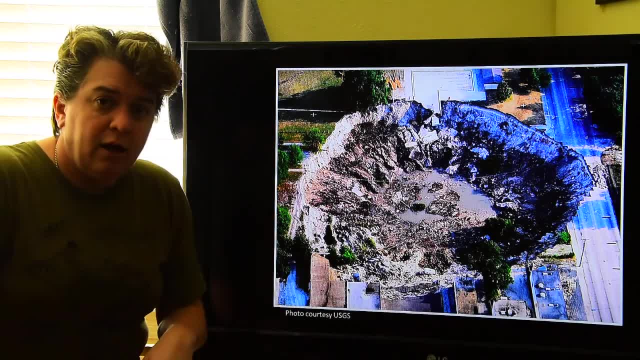 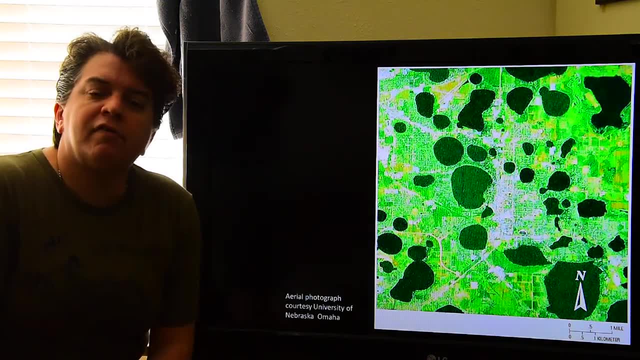 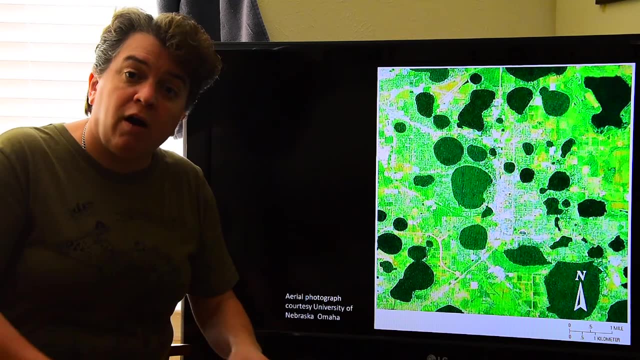 that is a truck with a camper shell on it, And this basically happened overnight. And these sinkholes, they're not a solitary feature, It's not like, oh, a sinkhole opened, it's done Because they form in certain types of bedrock. 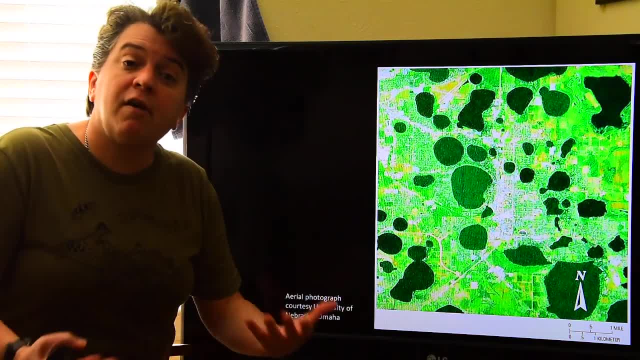 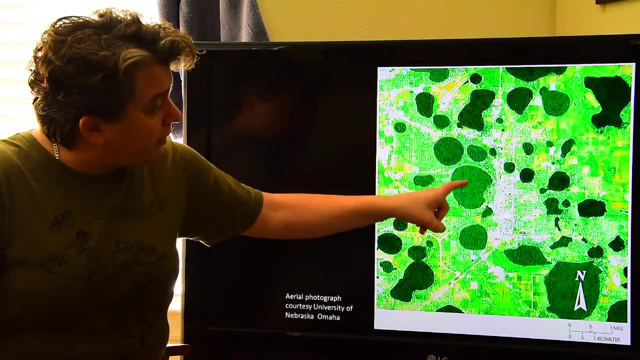 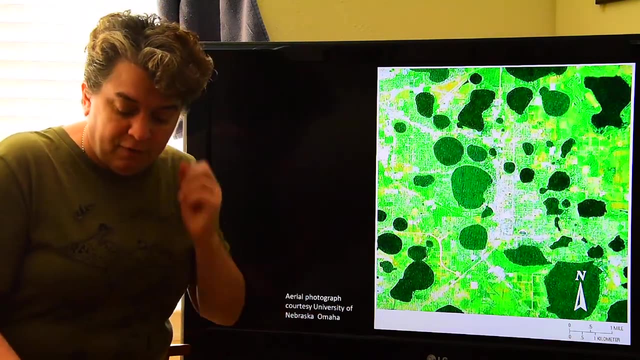 any place that has that bedrock is susceptible to a sinkhole opening. This is part of Florida, And each one of these dark areas is a little lake occupying a sinkhole, And that shows you that where you have one, you're likely to have another. 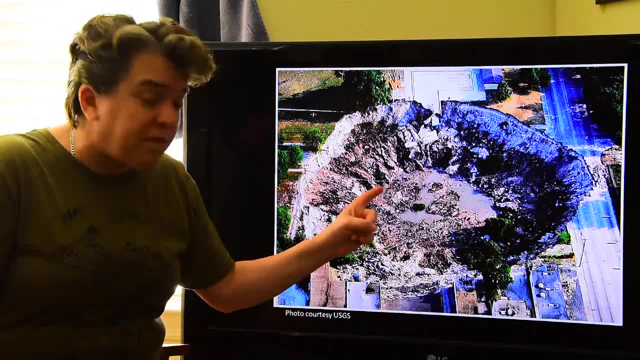 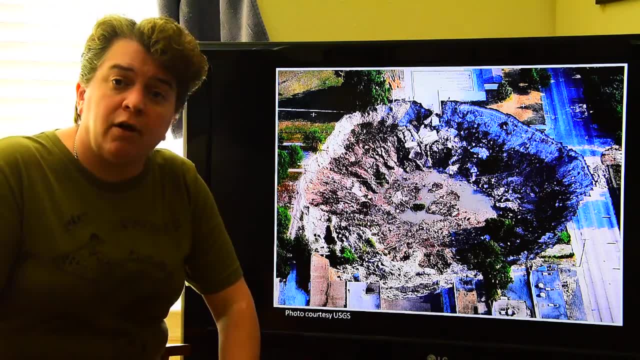 And, like I said, these things can be deadly. Imagine if that opened up under your house, And that does happen sometimes. A couple years ago, someone in Florida died when a sinkhole opened up under their house, If you want to watch one of these actually happening. 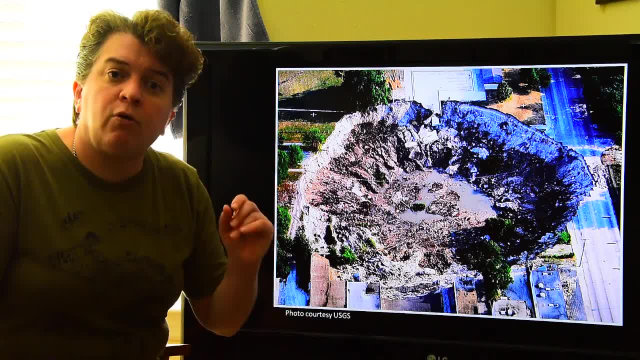 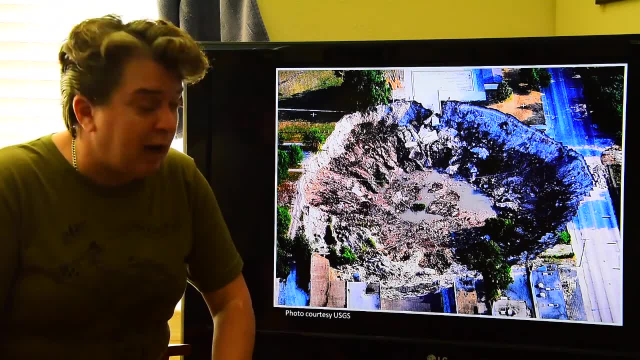 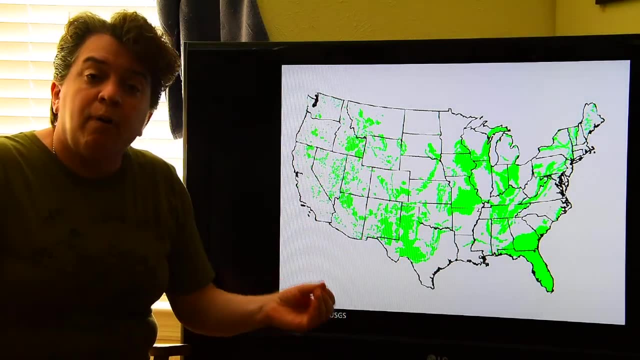 go to YouTube and in the search bar type in Corvette Museum sinkhole, And you'll get to see just how quickly a sinkhole can collapse. So in green on here, these are all areas that are underlain by soluble rock. So these are all places where you could have. 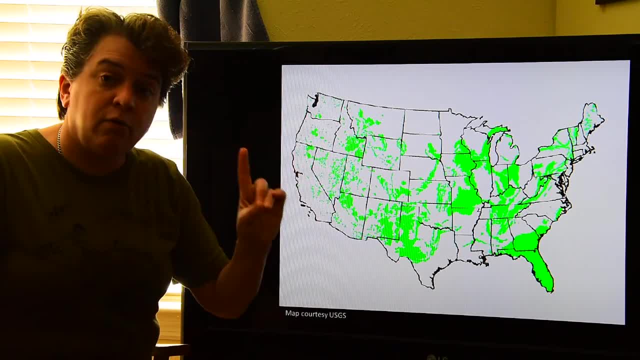 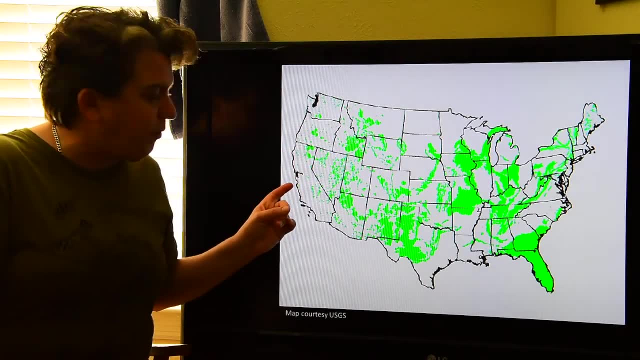 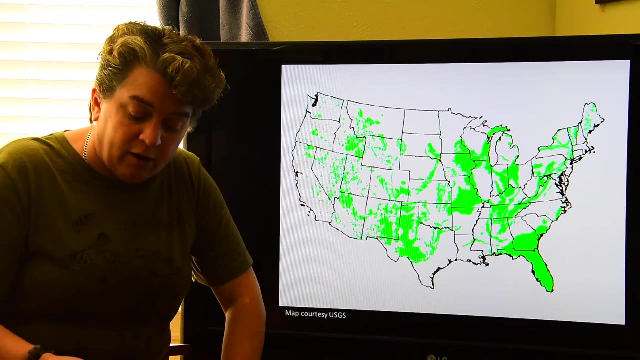 caves and karst topography forming and where you could have sinkholes. For once, California doesn't look too bad right. All the previous disasters seem to be focused on them. This time you really got to watch out in Florida, because almost all of the bedrock in Florida 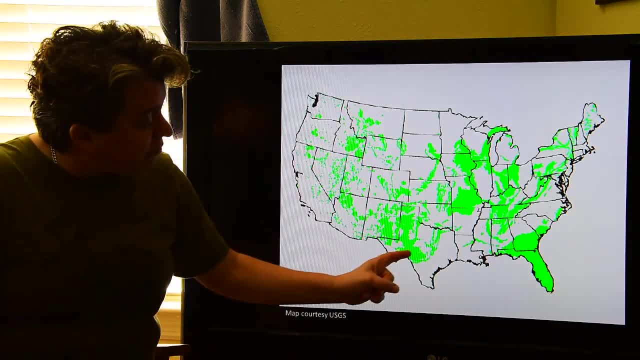 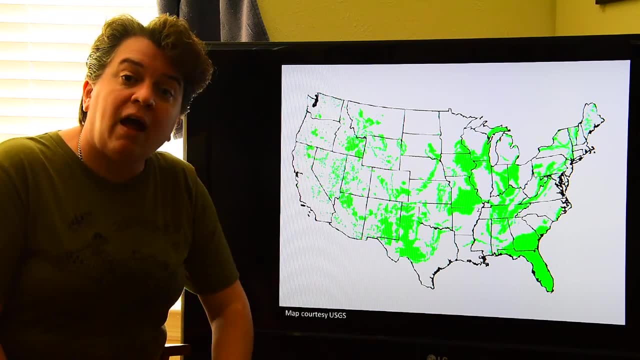 is limestone or dolomite. We also do have areas in Texas, and that's why you can go to parts of Texas and visit caves, because certain areas here do have limestone bedrock. So I just want to finish by showing you some really kind of neat areas.